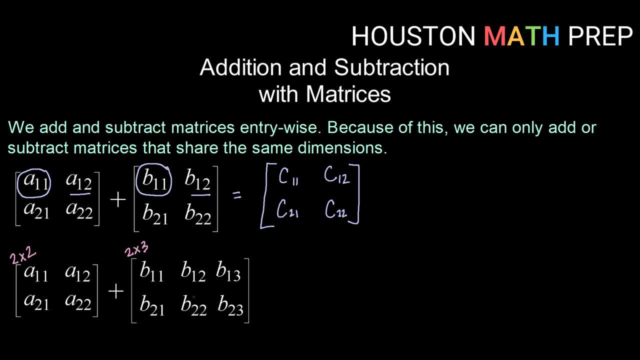 with a 2 by 3 matrix. When we got to entry b13, or the entry in row 1, column 3 of the second matrix, there is no item or entry from the first matrix to add that with. Therefore this addition. 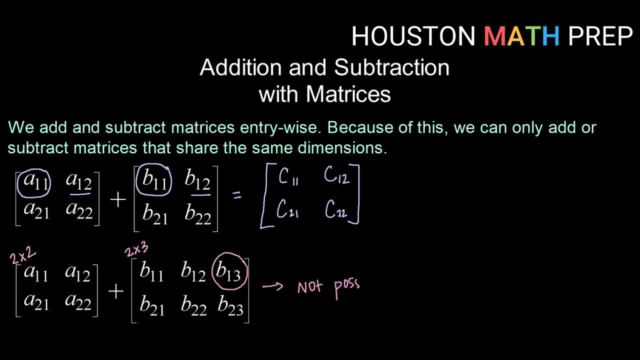 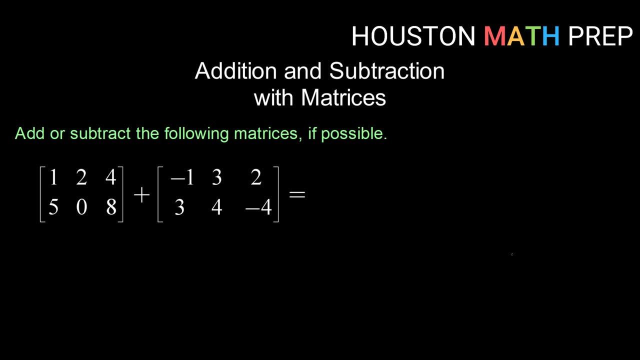 is not possible. So if we are adding or subtracting matrices, they have to have the same dimensions. Okay, let's check out some examples of this process. So here we want to add or subtract these matrices if possible. So first we want to check. is it possible? Well, check to see. 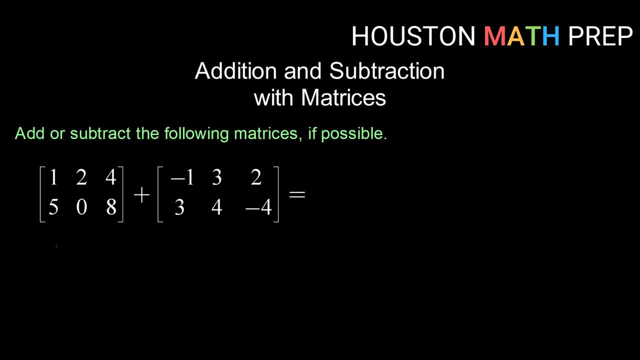 if your matrices have identical dimensions. So our first matrix has two rows by one, two, three columns, So we have a two by three. Our second matrix again has one into the two rows by one, two, three columns, So we're trying to add a two by three with a two by three. 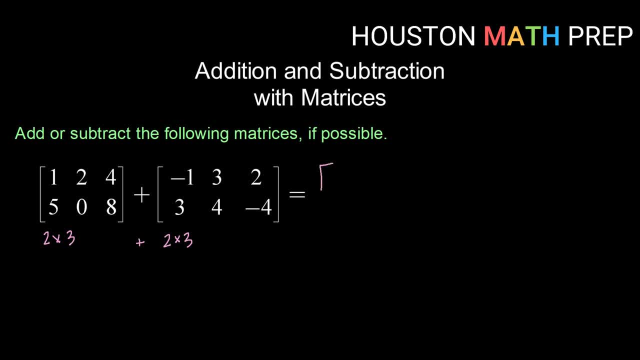 Since our dimensions match, we can do that and also our result will be a two by three. So we can kind of set up for that. So to fill in this entry in row one, column one, we're going to take the entry from the first matrix in row one, column one and add it with the second entry. 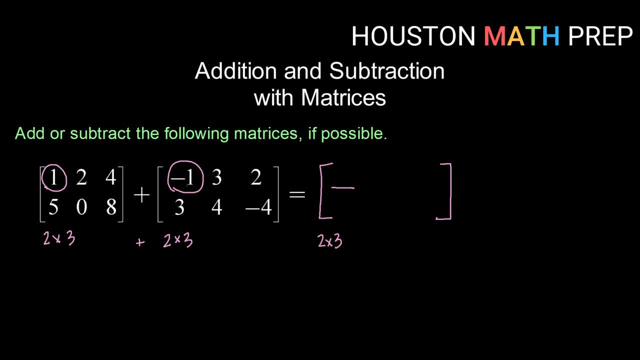 or sorry, the entry in the second matrix in row one, column one. So that would be one plus negative one, which is zero For our next entry in that row. so, row one, column two: same idea: Two plus three makes five. Continuing this process, four plus two makes six. 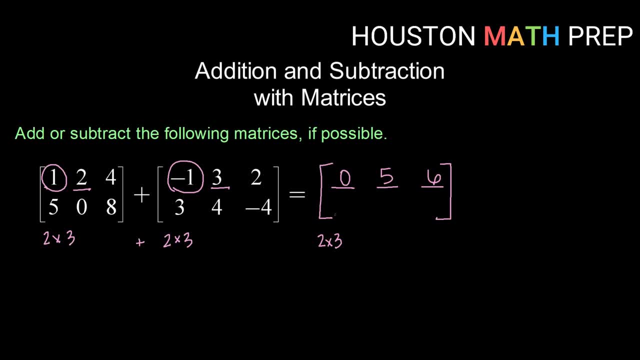 Four entries in row 1,, column 3.. 5 plus 3 makes 8 for row 2,, column 1.. 0 plus 4 makes 4 for row 2,, column 2.. And then, last but not least, in row 2,, column 3,, we have 8 plus. 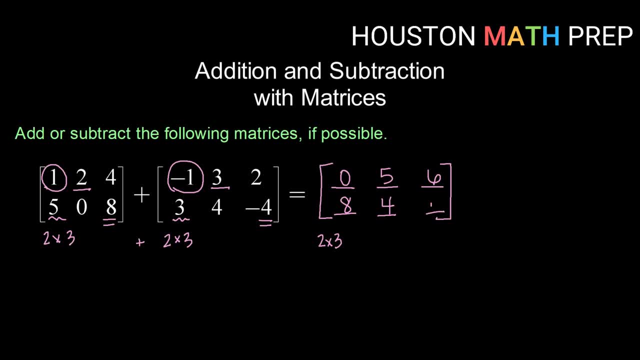 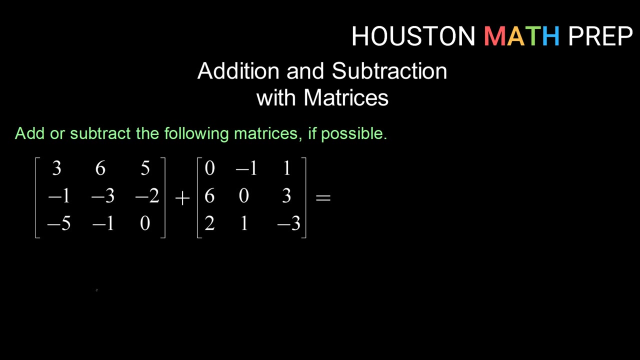 negative 4, which is 4.. So here is the result of adding this first 2x3 matrix with this second 2x3 matrix. All right, let's check out another one. Add or subtract the following, if possible, so that if possible says check the dimensions. So here in our first 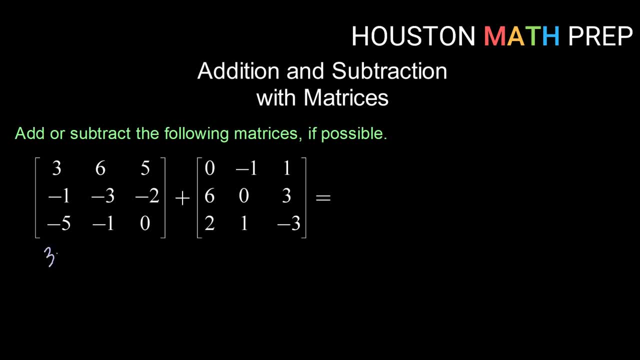 matrix. we have one, two, three rows, so this is a three by one, two, three columns. so we have a three by three and we are trying to add to that another. let's see one, two, three rows by one, two, three columns. so we have a three by three adding to a three by three. so since those dimensions match, 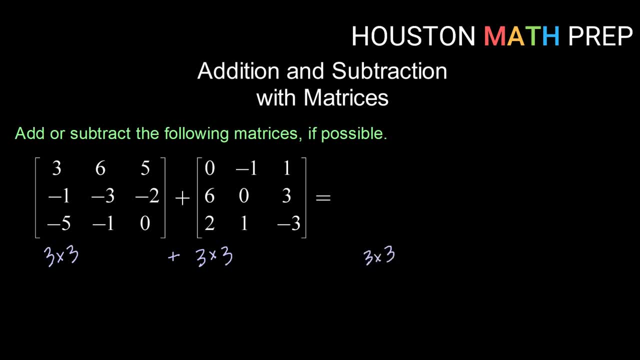 this is possible and our result will have the same dimensions. we will have a three by three to match. so three rows with three entries each. all right, to fill in row one, column one, we'll add the entries from each matrix in that spot. so three plus zero makes three. continuing along row one, six plus. 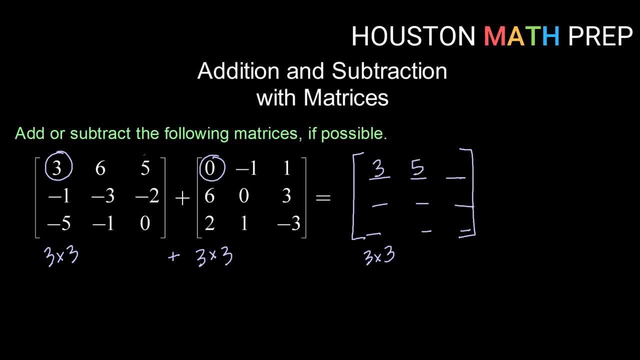 negative one makes five. continuing along row one, five plus one makes six. since we've completed row one, let's move to row two, taking the first entry in row two from each matrix. negative one plus six is five. negative three plus zero is negative three. negative two plus three is positive one and that means we've finished row one. we will be Gemini four by five. 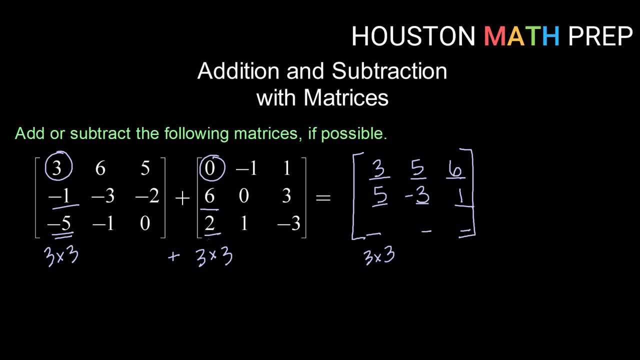 row 2, finishing up in row 3, negative 5 plus 2 makes negative 3, negative 1 plus 1 makes 0, and 0 plus negative 3 makes negative 3.. So here is our solution to a 3 by 3 plus this 3 by 3.. 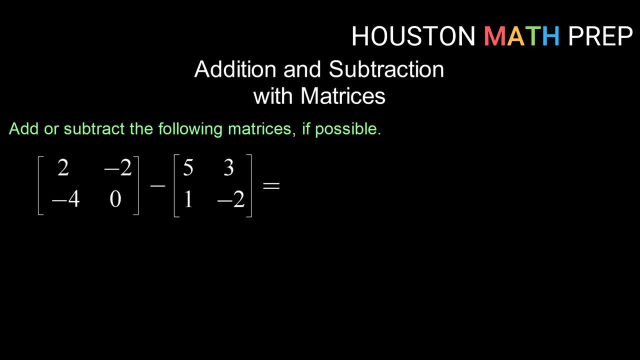 All right. in our next example let's take a look at what, if anything, is different if we are subtracting matrices. So really the only difference here is the operation. We still first need to check to see that our matrices share the same dimensions. So here we have a 1, 2 by 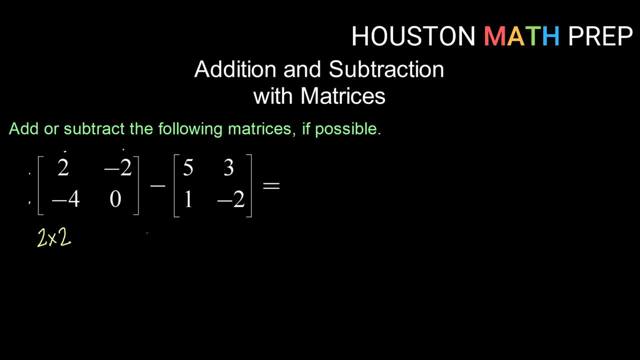 2 column, so a 2 by 2, and we are subtracting this one has 1, 2 rows by 1, 2 columns, so a 2 by 2 minus a 2 by 2, that is possible and it will result in a 2 by 2.. 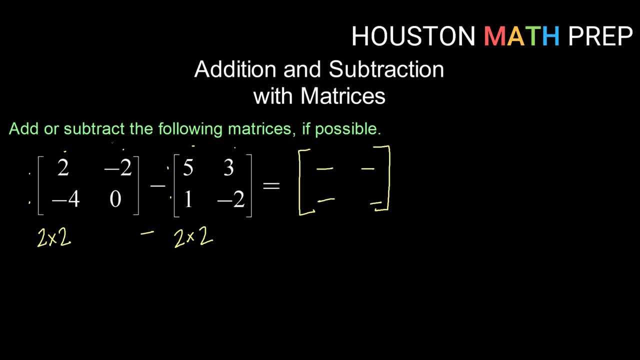 All right. so now we're going to subtract the first first matrix minus the second entry-wise. So for row 1, column 1, we'll take 2 minus 5, that will give us negative 3 in row 1,. 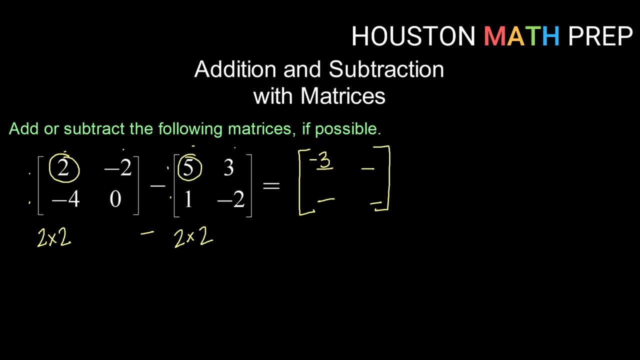 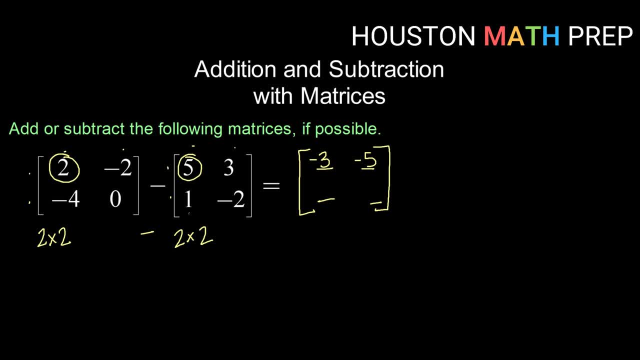 Moving on to row 2, negative 4 minus 1 will make negative 5 for row 2,, column 1.. And finally, for row 2,, column 2, 0 minus negative 2, remember, minus a negative is like plus. 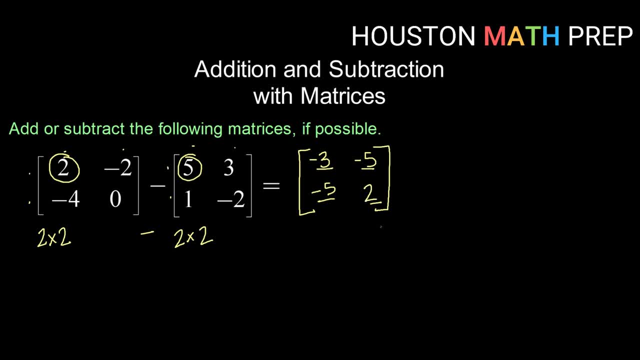 so that'll give us 2.. All right, so there we have it. Subtraction looks a lot like addition. just remember that we are subtracting that second value. All right, here's another one. Add or subtract the following matrices if possible. So check out your dimensions, see if you can do it. 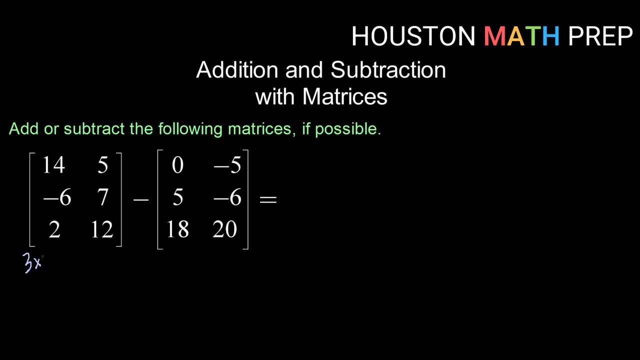 This first one is a 3 row by 2 column, so 3 by 2 minus second one, we have 3 rows, 2 columns, so we can do this operation and it will result in the same size matrix, another 3 by 2.. So let's do this by rows. 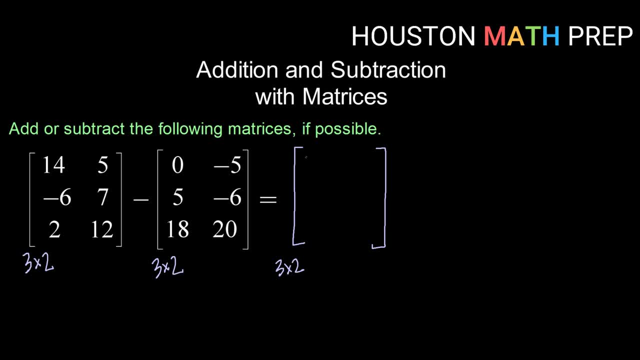 14 minus 0 in row 1, column 1 gives us 14.. Row 1, column 2, 5 minus negative 5, remember: minus a negative plays like a plus, so that would be 10.. Column 2, negative: 6 minus 5,. 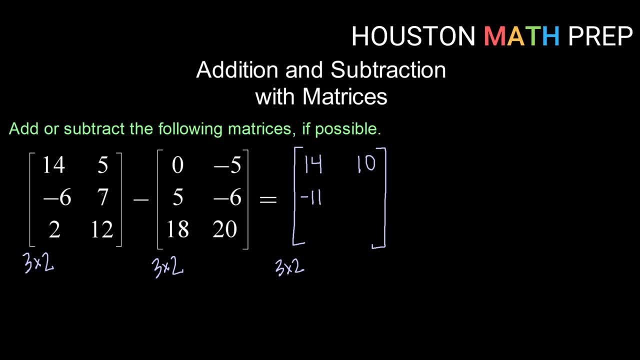 will give us a negative 11.. 7 minus negative 6, minus a negative acts like a plus, so that will be 13.. 2 minus 18 is a negative 16 for row 3,, column 1.. And last but not least, row 3,, column 2,. 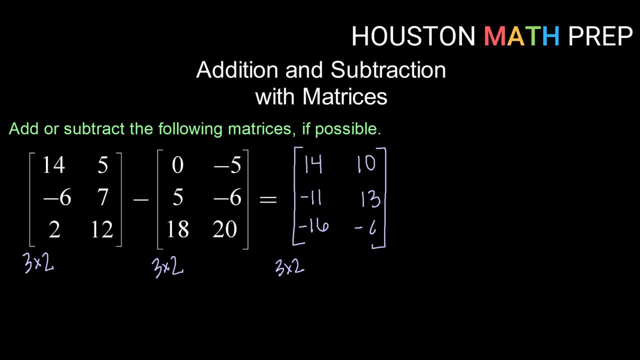 12 minus 20 makes a negative 8.. So here's our result, our 3 by 2 answer matrix. All right, final example: Add or subtract if possible. So let's check it out. Check our dimensions. We have 1,, 2, 3 rows here, by 1, 2, 3, 4 columns, so a 3 by 4 in our first one. 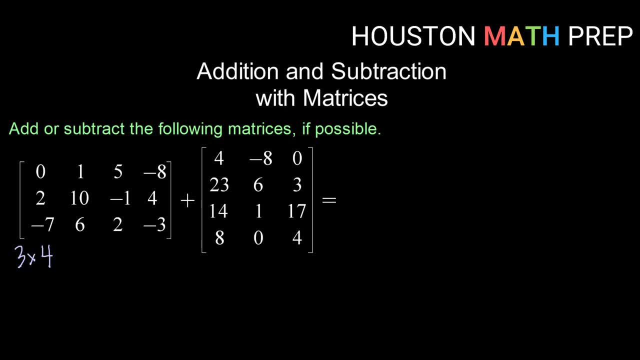 And we're trying to add to that a 1,, 2,, 3, 4 rows by 1, 2, 3 columns, so a 4 by 3.. Here, although the dimensions share the same numbers, the number of rows is different and the number of columns is different. So these: 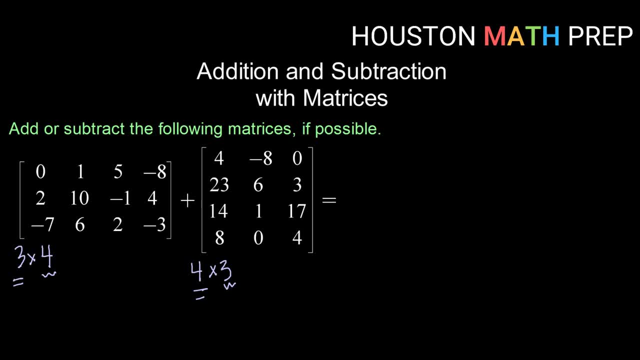 two matrices are not the same size and therefore they cannot be added, So this is not possible. All right, guys, that does it for this video on addition and subtraction with matrices. Until next time. we'll see you later.